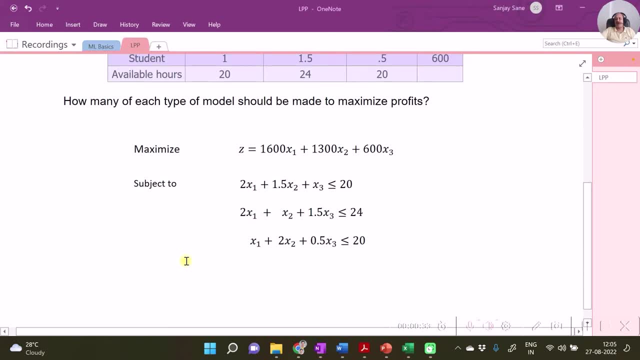 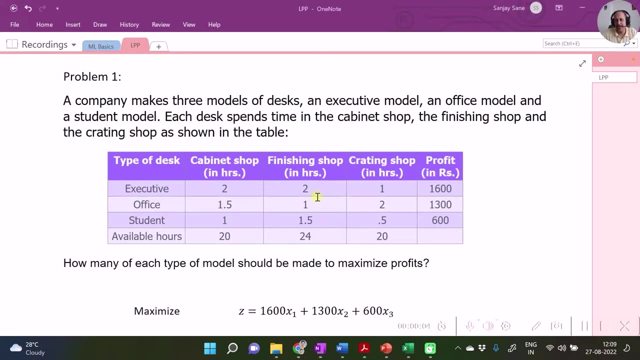 maximized Over here. as you see that I have formulated this problem, We need to first of all do spreadsheet modeling for this problem before we use the option of solver. So to start with, let us have the three variables specified in our spreadsheet, namely executive. 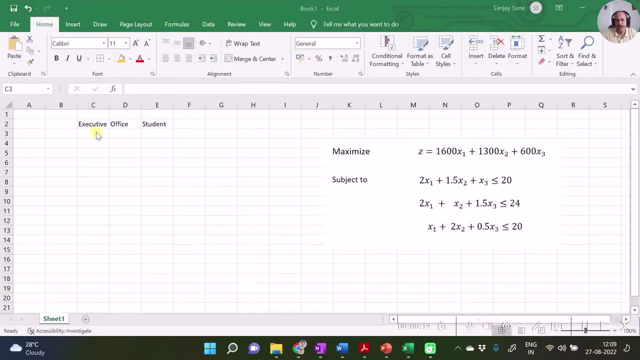 office and student. Now we require to specify the profits accordingly for this. So this is per unit profit, As I am specifying here. So it is respectively 1600 for first product, 1300 for second product and 600 for third product. Over here we need to place the values actually. So our solution: 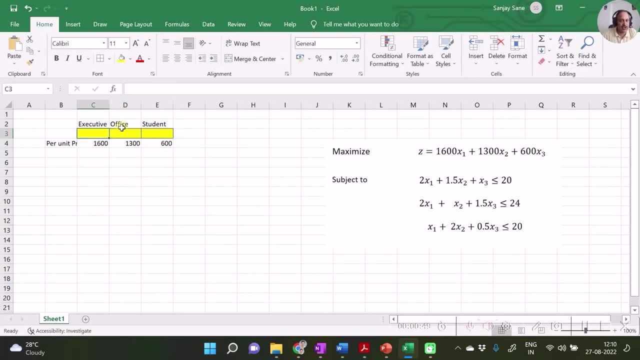 is going to be in the cells C3, D3 and E3 respective. Let us first of all calculate the maximization function, which is 16 into X1,, 13 into X2 and 600 into X3. Now the best function in Excel, for this can be some product which will have. 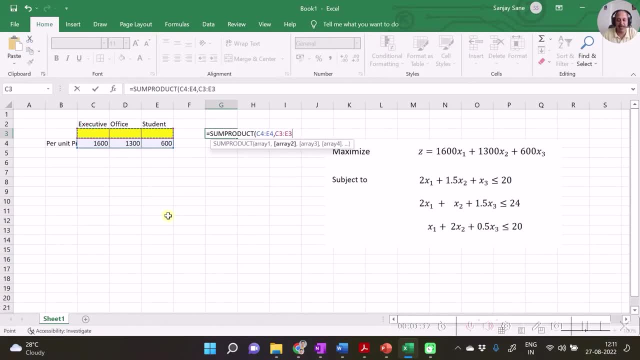 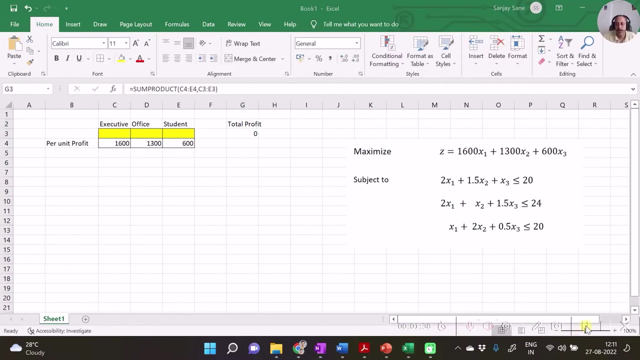 this multiplied with this- we usually call it mathematics- as dot product. You can test well over here whether you are getting correct value or not. you can keep it blank also. so here comes our total profit. now, having done this, we need to arrange the data for these. 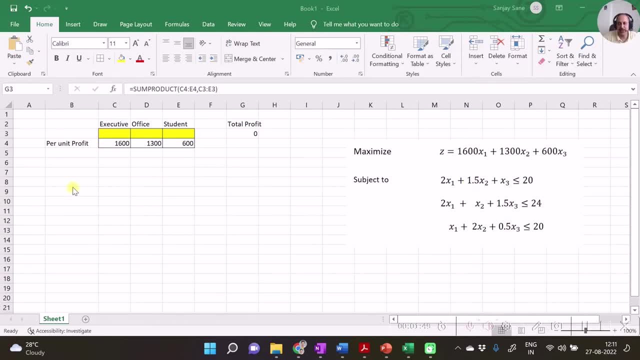 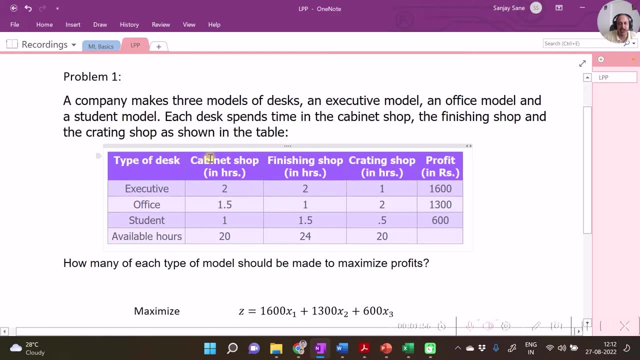 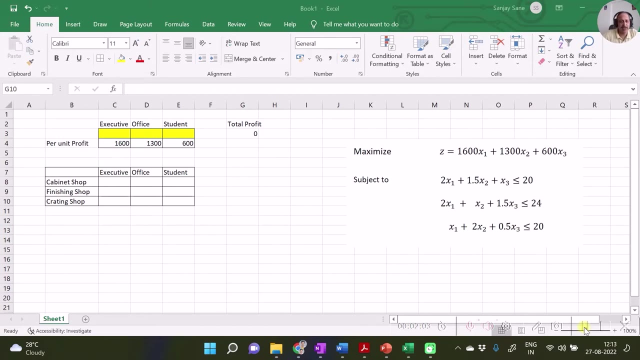 three constraints in a separate table. let's do it so. the first constraint which is there in our problem, basically the first constraint, is of cabinet shop, finishing shop and creating shop. in this way we require to arrange. this data means we are actually going to enter now 2. now for the first constraint. it is 2x1 plus 1.5 into x2. 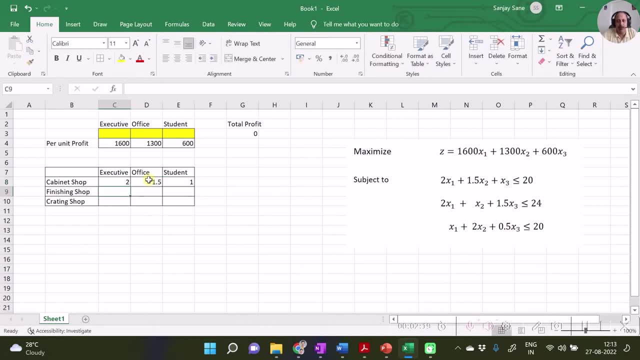 1.5 into x2 and 1. well, now, this upper limit which is specified over here has to be also in one particular column. let us name this column as available hours. well, it will be. it will be 20, 24 and 20 respectively for three constraints and accordingly, let us see that. 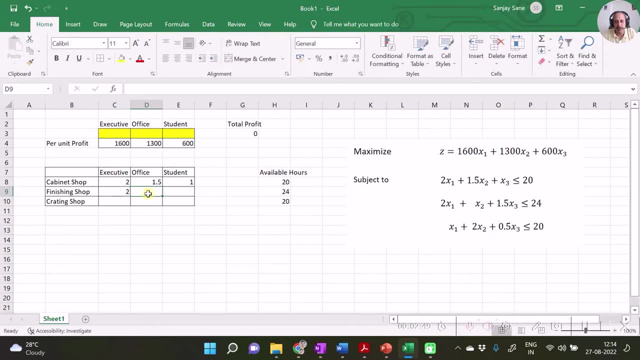 enter the values for these three other constraints and also for the third constraint. having done this now, first of all, we need to have one more column which actually specifies the left hand side of our equations or inequalities. i can say it is two into x1, so what is x1? 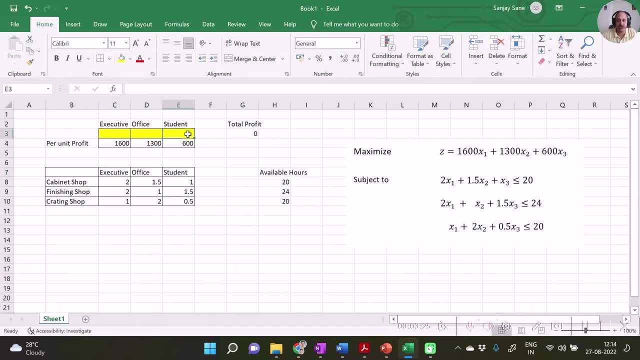 over here. this is x1 cell, this is x2 cell and this is x3 cell. so hence the way we have calculated some product over here, in the same way we are going to calculate some product for these cells. so some product, so two x1 plus one point five into x2 plus x3 and x4. 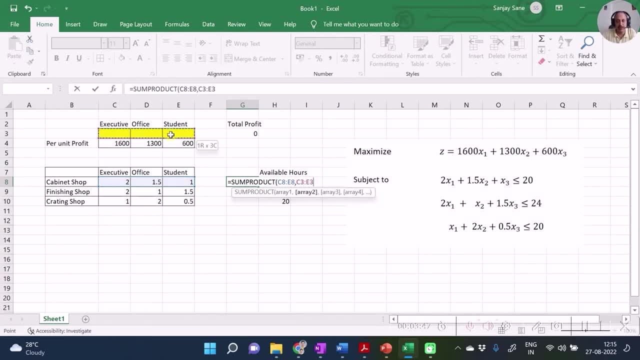 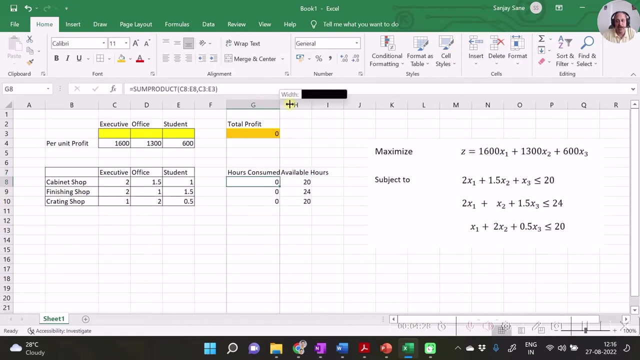 x3 is going to be implemented with this sum product. so, basically, sum product is going to complete our left hand side of all of our inequalities which we have specified here. accordingly, the last one. well, let us name this column as hours consumed or hours utilized, whatever. so these are going to be our hours consumed and these are going to be our hours. 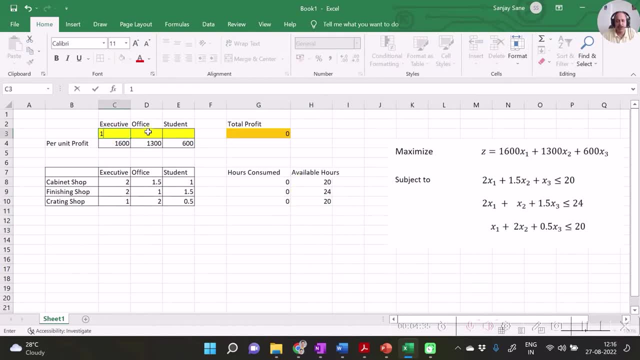 available Now. we can put some values in this and see for the for any feasible solution. so you can. you can anyway change the values and you can anyway get the changing other cells like total profit. but what we intend to do is that we want the values of executive office and student like yc3, d3. 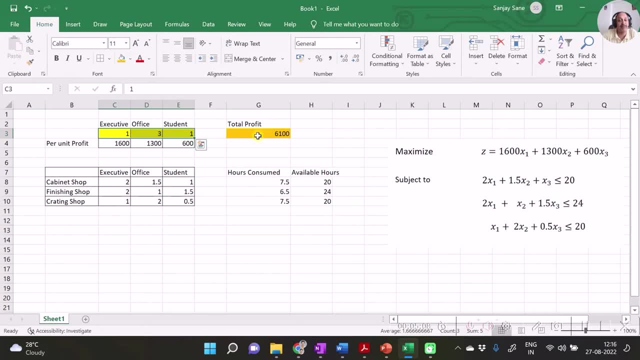 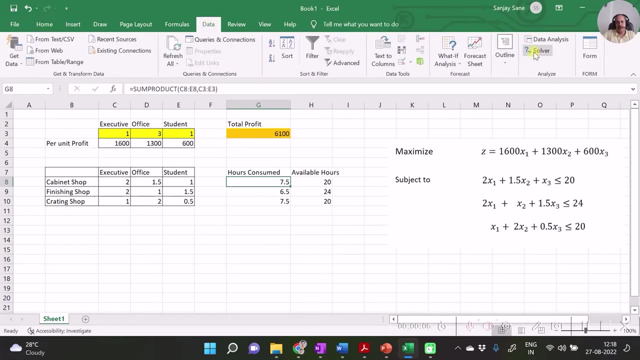 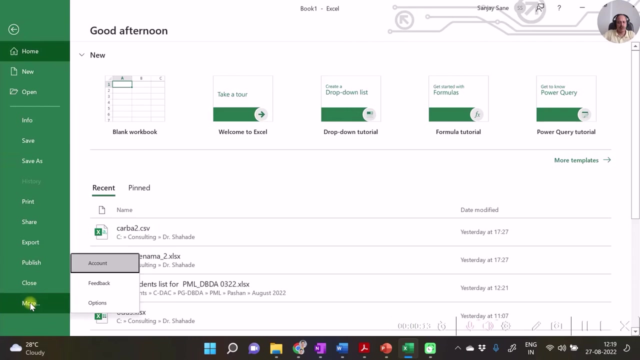 and e3. In such a way that the total profit will be maximized with the constraints followed. how can we do that? let us see over here: we need to basically enable the button solver in the data reaper for doing that. go to file, then go to options. well, over here my version of 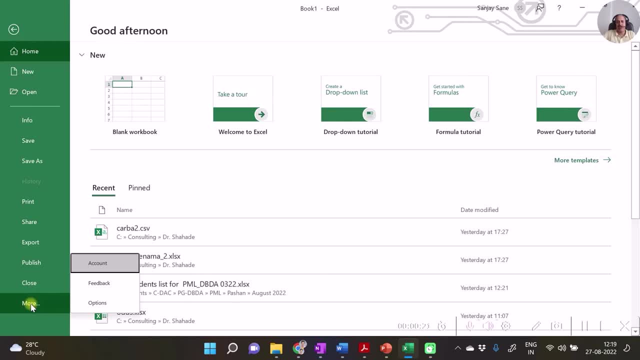 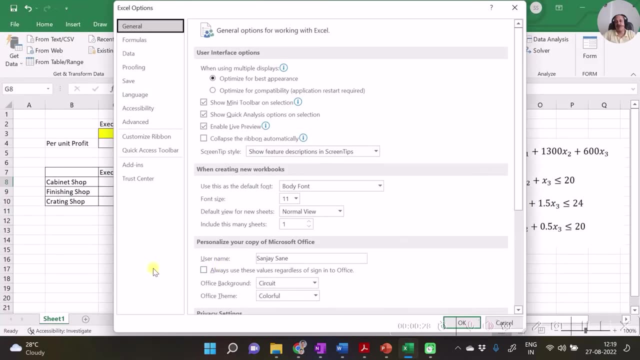 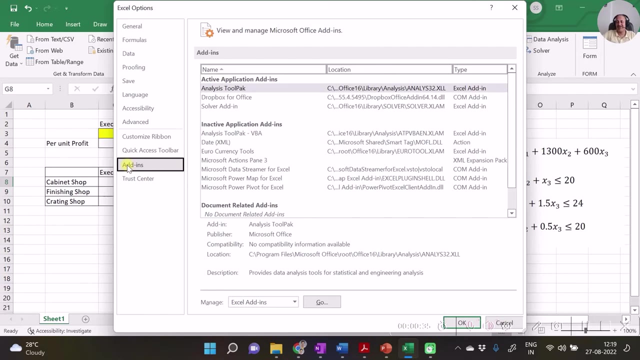 offices. If your version is earlier than, please search for options. first of all, once you search for options, the Excel options dialog box gets open. go to add-ins, because basically that solver is an add-in, so go to add-ins and then in the manage add-ins, in the manage add-ins. 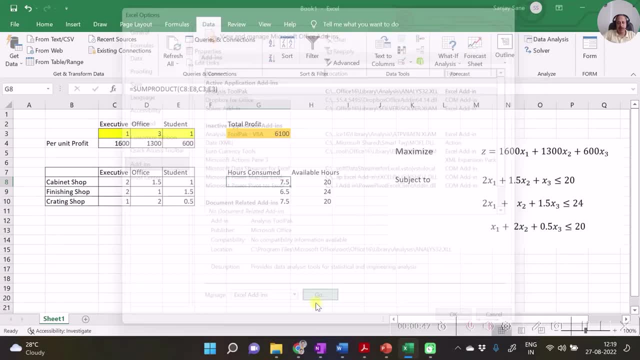 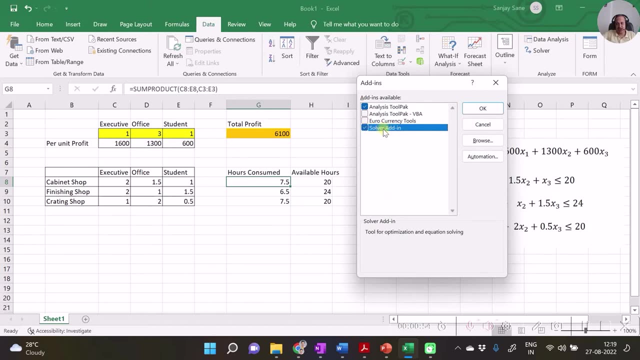 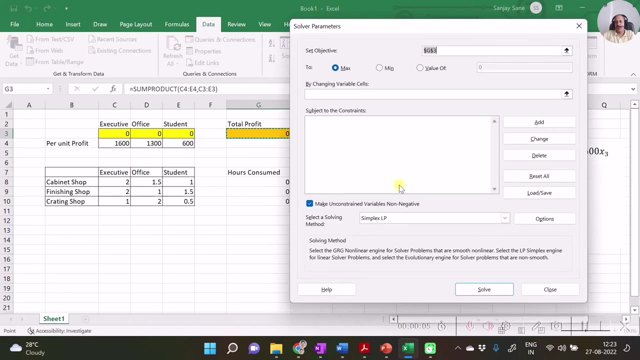 you see, please select the excel add-ins, click on go button and ensure that. ensure that your solver add-in checkbox is is checked. now click on ok so that your solver button gets enabled in the data. so to begin with I click on solver button. ensure one thing: while you you do anything with solver: 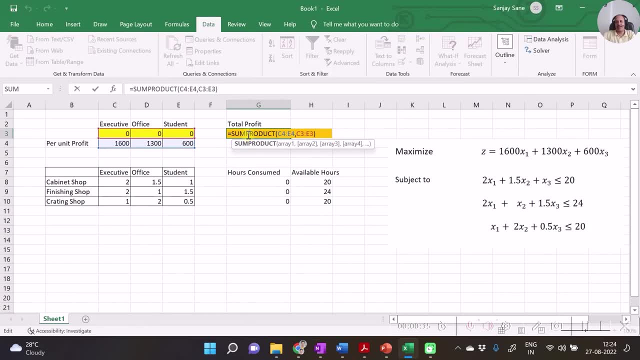 ensure that your total profit cell is ready with the total profit, because this is the cell where your total profit is going to be evaluated. okay, so please ensure that total profit the you have filled in the proper formulae. also, ensure that in the hours consumed you have filled in the proper formulae so that 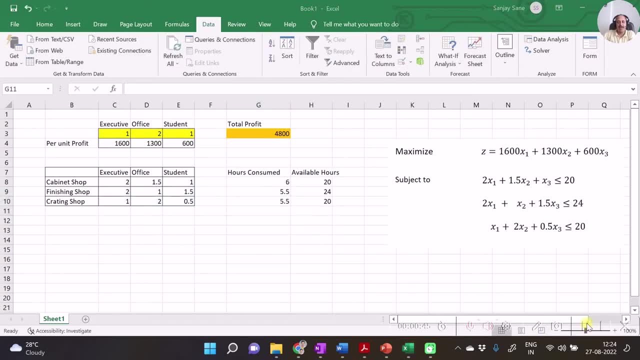 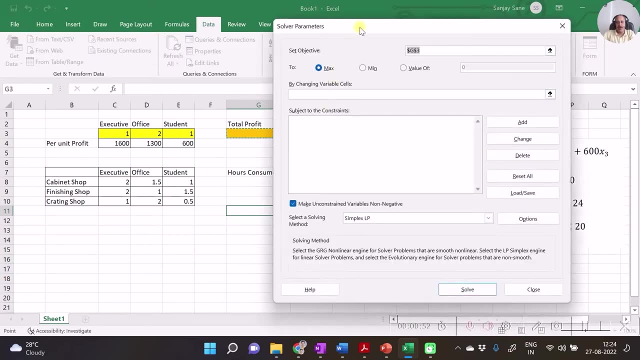 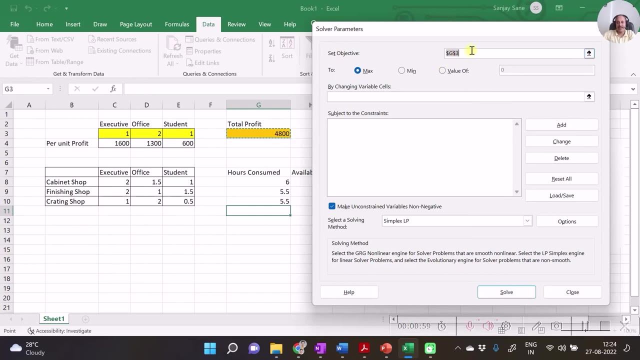 your values can get calculated correctly. now, having set all this up over here, well, what I am going to do is I want to maximize the profit. so maximization profit, maximization cell is going to be G3. by changing the cells. which one? by changing these three cells, because these three cells are the cells. 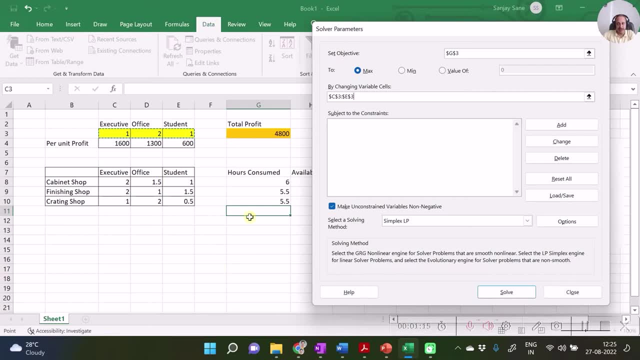 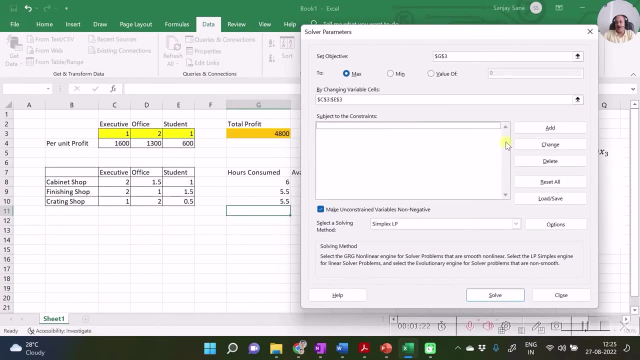 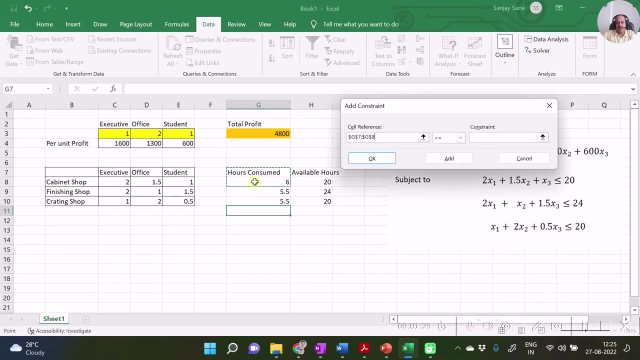 by which we have set all the formulae for x1, x2, x3, isn't it now? having done this, having done this, go to the constraints. on to the constraints, click on add and this is your LHS. this is going to be your LHS and this is going to be your RHS. so the formula of 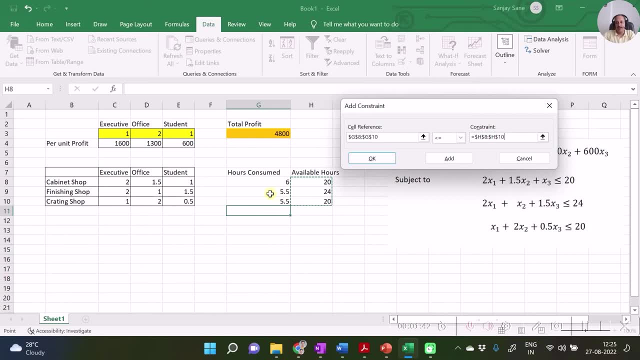 hours consumed are. I am going to be there in these cells, and this is the constraint upper value: ensure the proper equality or inequality of this. if, in case, your problem is filled with inequalities, with less than also, greater than also, then you will have to maintain separate constraints. 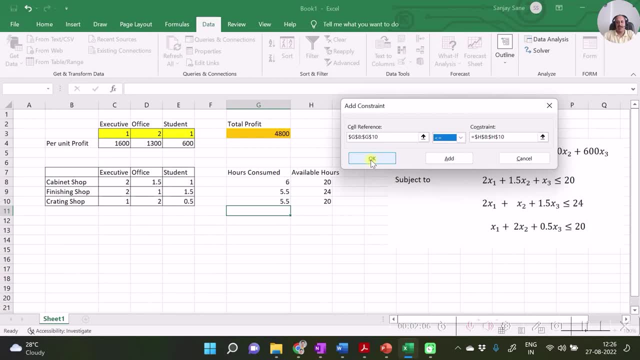 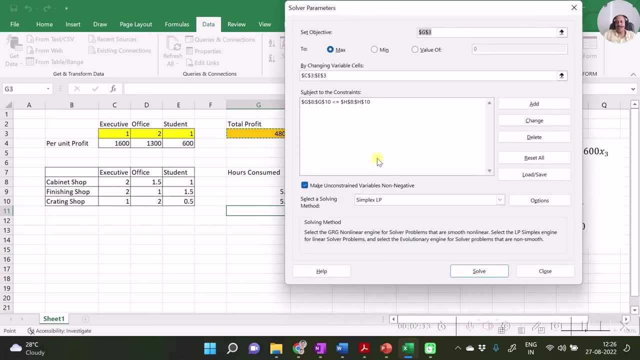 for that. having done this, I click on ok button. as we have less than or equal to inequality, then if you want to solve this problem with simplex linear programming problem method, then opt for simplex LP or you can opt for nonlinear. over here I am opting for simplex. 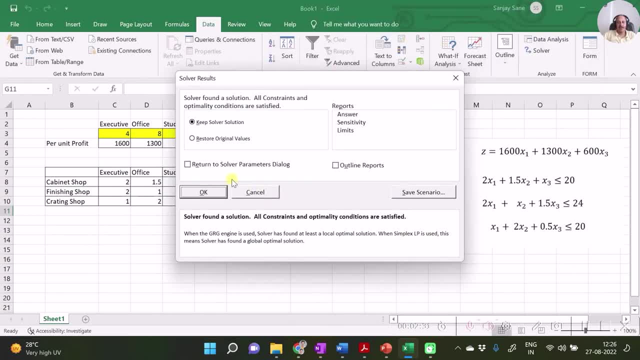 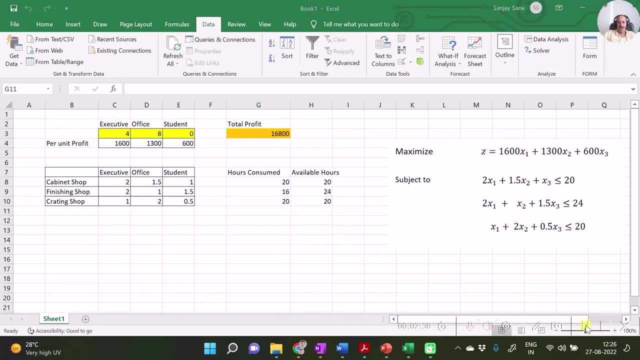 LP and I am clicking on solve. now, clicking on ok, we see that we get the solution. hence, what solution have we got? if we manufacture four pieces of executive type, eight pieces of office type and no piece of student type, then our profit is going to be the maximum profit, with the constraints followed. 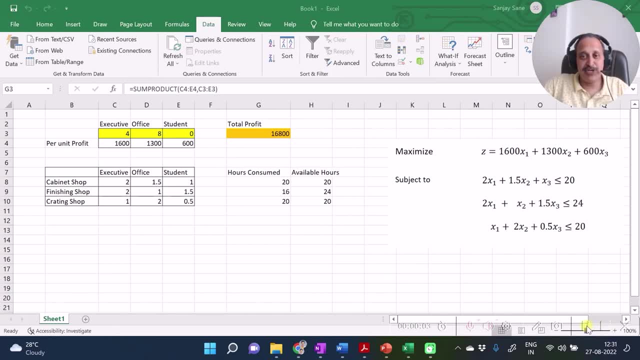 thanks for watching this video. if you like this video, please click the like button, and for updates from me, please subscribe to my channel. thank you.